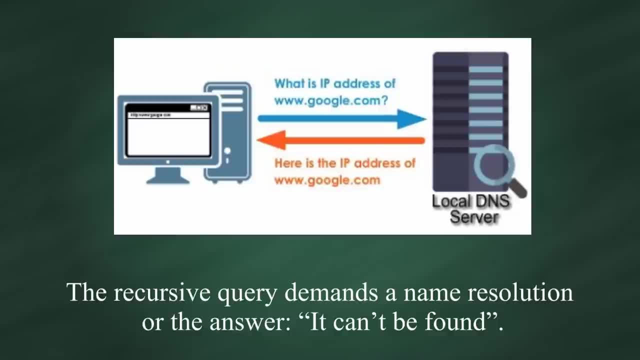 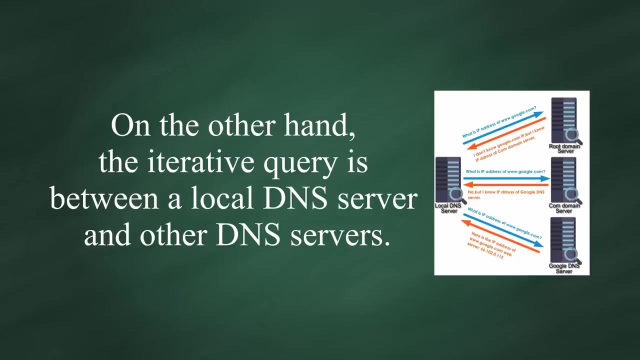 their definitions. first, The recursive query demands a name resolution or the answer. it cannot be found. The recursive query is between DNS client and its local DNS server. On the other hand, the iterative query is between a local DNS server and a local DNS server. 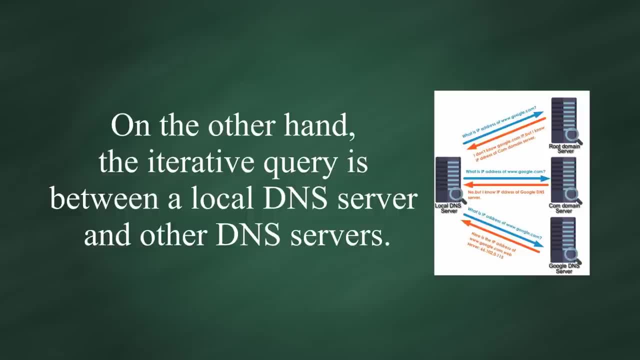 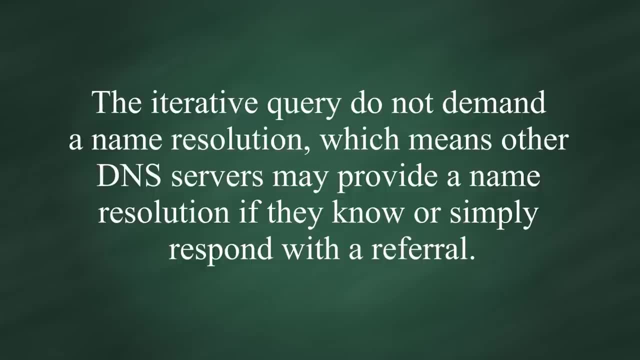 The iterative query is between a local DNS server and a local DNS server. The iterative DNS server and other DNS servers, The iterative query do not demand a name resolution, which means other servers. other DNS servers may provide a name resolution if they know or. 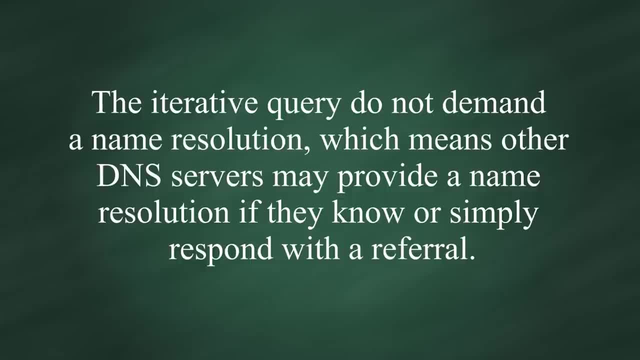 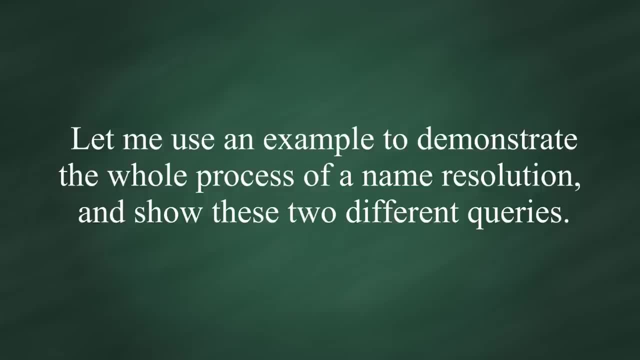 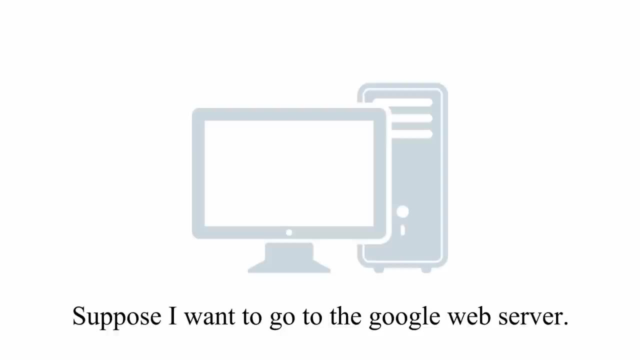 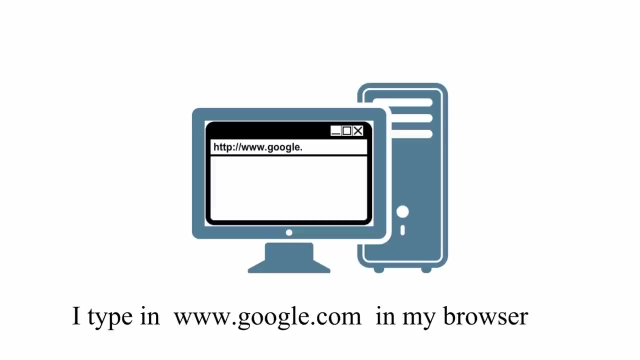 simply respond with a referral. Let me use an example to demonstrate the whole process of name resolution and demonstrate these two different queries. Suppose I want to go to a Google web server. I type in wwwgooglecom in my browser and hit enter My web browser. 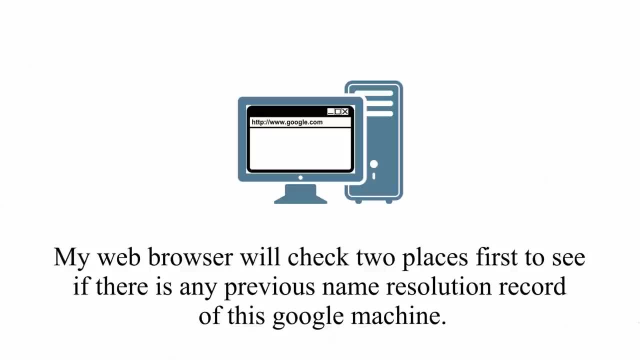 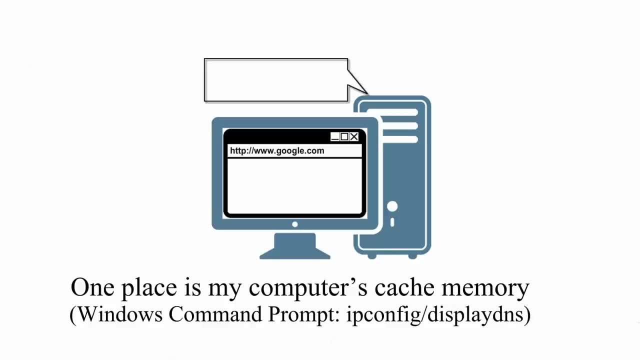 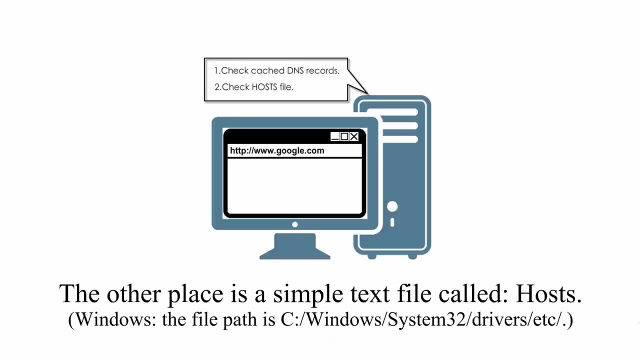 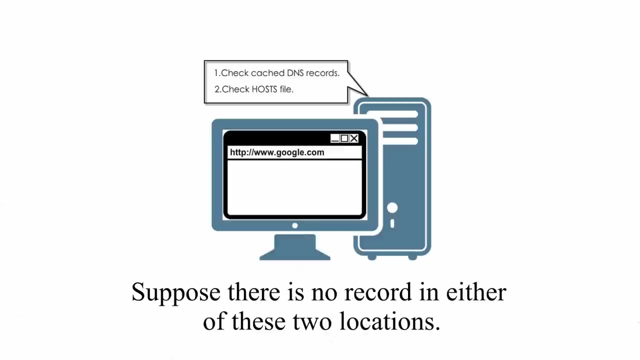 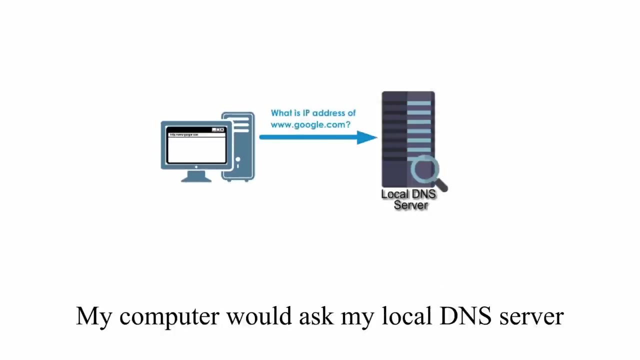 will check two places first to see if there is any previous name resolution resolution record of this Google machine. One place is my computer's cache memory. The other place is a simple text file called hosts. Suppose there is no record in either of these two locations, My computer would ask my local DNS server. I want to know IP address of W2. 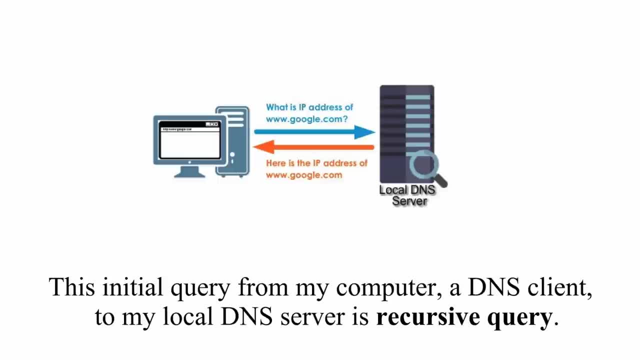 code I type in W2.googlecom. This initial query from my computer, a DNS client, to my local DNS server is recursive query Because my computer demands a clear answer. to resolve a name is the responsibility of my local DNS server. Let me assume that my local DNS server here has a name resolution value in the root of my domain name. I am sorry that this is not correct. I will need to query it again. This is my local DNS server, the same as my local DNS server. I want to know the name of my. 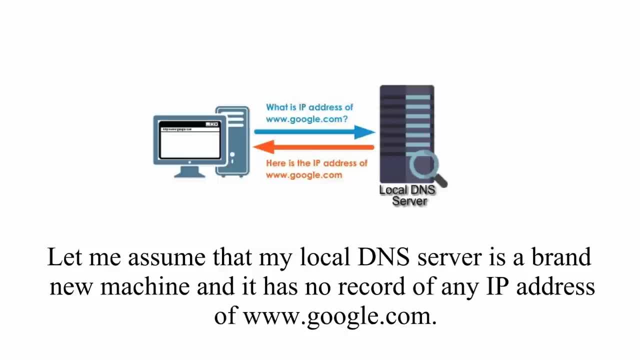 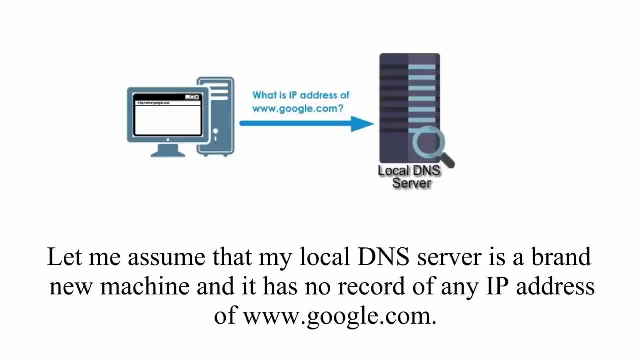 user as my local DNS server. I want to know the name of my local DNS server. I want to know the name of my DNS server and I want to know, possibly, the number of DNS server name and local DNS server is a brand new machine and it has no record of any IP address of wwwgooglecom. 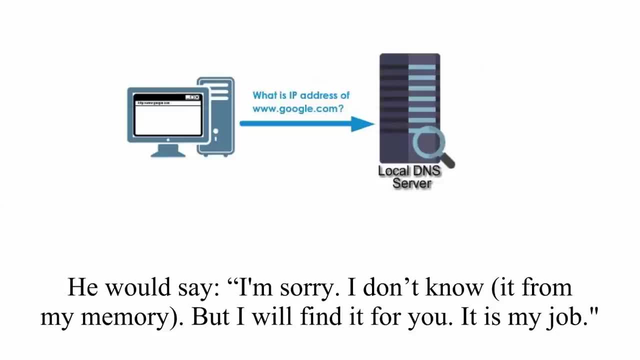 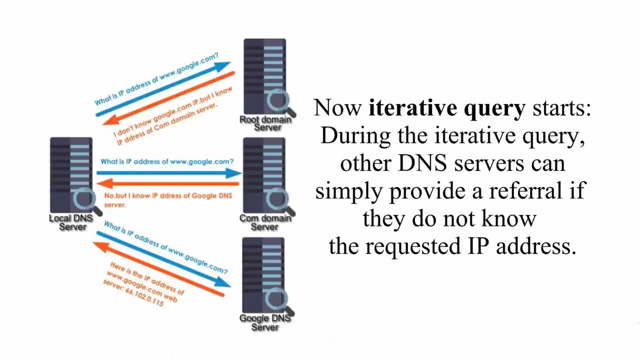 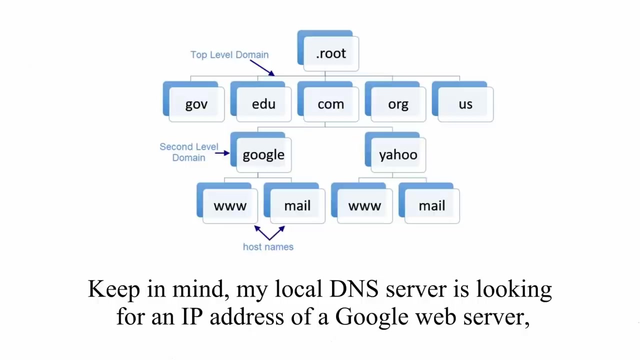 he would reply. I'm sorry, I don't know, but I will find it for you because that's my responsibility. Now the iterative query starts. remember, during the iterative query, other servers can simply provide a referral if they do not know the IP address of wwwgooglecom. 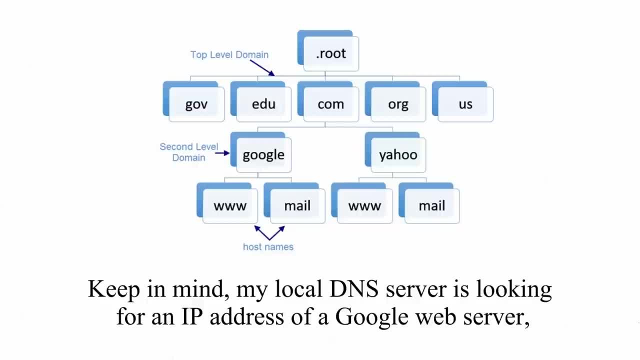 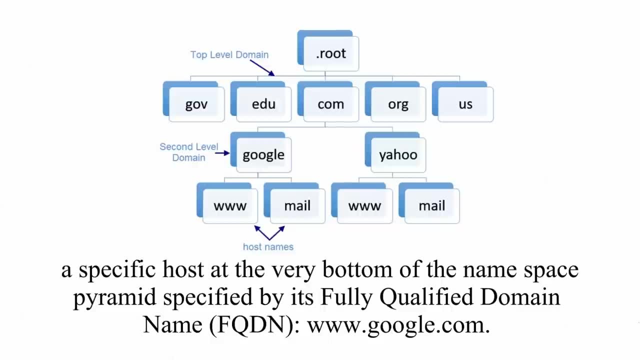 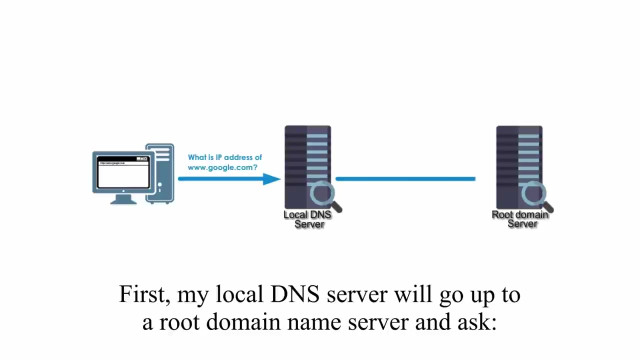 Keep in mind, my local DNS server is looking for IP address of Google web server, a specific host At the very bottom of the namespace pyramid specified by its fully qualified domain name: wwwgooglecom. first, my local server will go up to the root domain server, because everybody 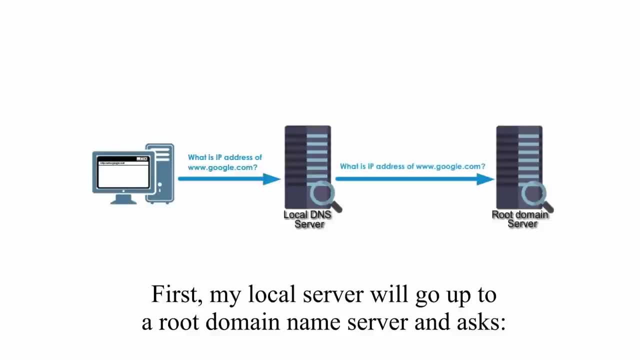 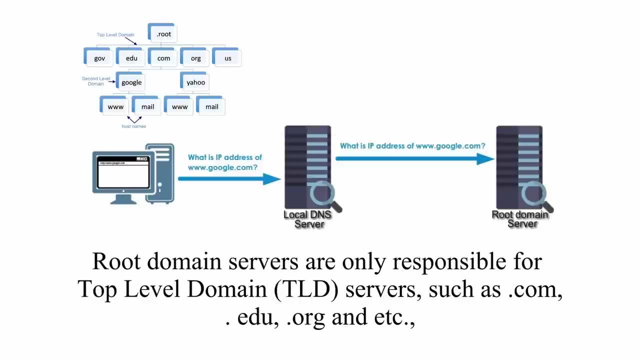 knows root domain server and asks: do you know what's the IP address of wwwgooglecom? Yes, wwwgooglecom. So root domain servers are only responsible for the top level domain servers such as com, edu, org, etc. 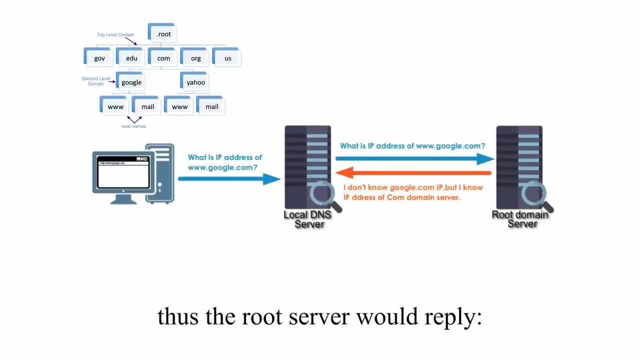 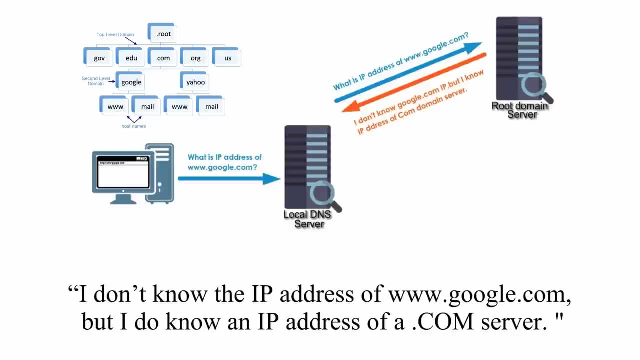 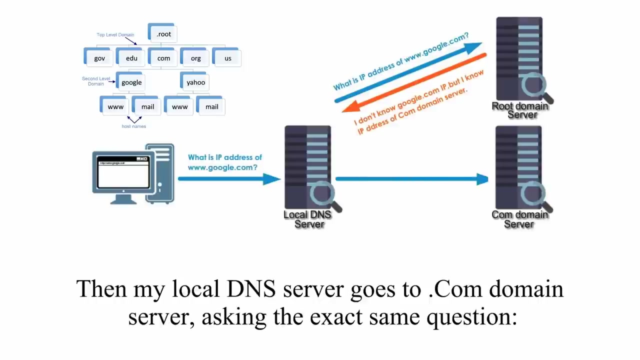 Thus the root domain server would reply. I don't know the IP address of wwwgooglecom, but I do know an IP address of com. Next, ladies and gentlemen, Next com server. Here the root domain server gives a referral, Then my local DNS server goes. 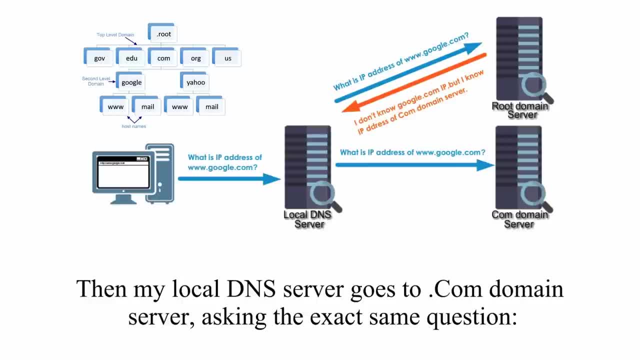 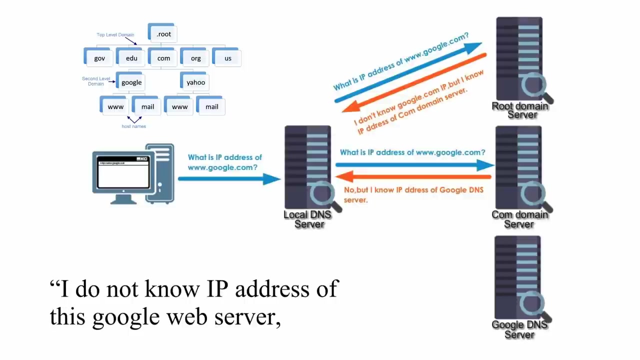 to the com server and asks the exact same question: do you know what is the IP address of wwwgooglecom? The com server would reply: I don't know the IP address of this Google web server, but I do know the IP address of the Google DNS server under me. You can. 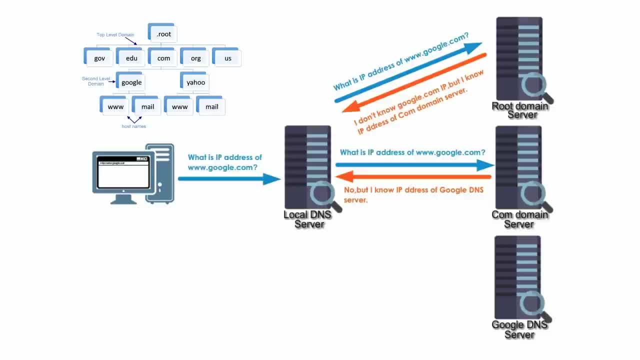 ask him Here. the com server is open. Also, give a referral. Well, my local DNS server never give up. He finds the Google DNS server and asks the exact same question: do you know what is the IP address of wwwgooglecom? 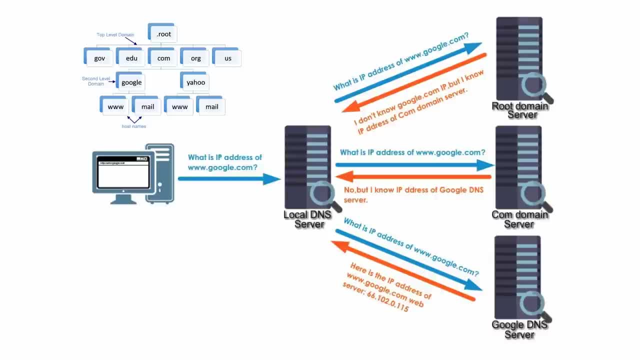 Well, this time the answer is yes, because Google DNS server shouldn't know any Google host IP address. His response is like this: Here is one IP address you can use. Once my local DNS server gets its IP address, it informs my computer, which will use this IP address to talk to. 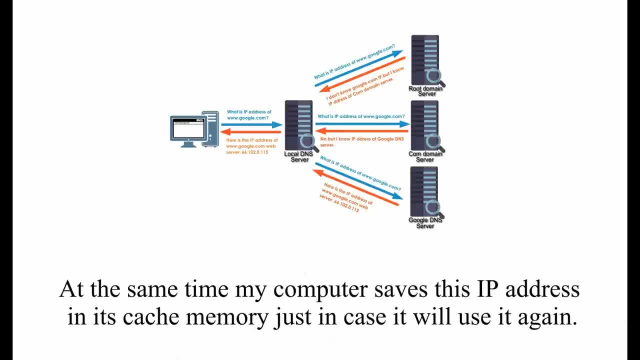 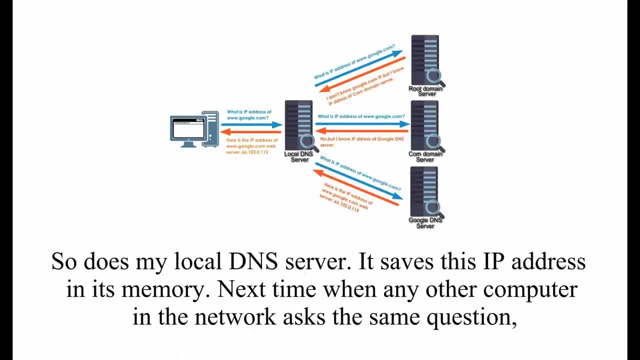 the Google web server. At the same time, my computer saves this IP address in its cache memory, just in case it will use it again. Well, that's it. Thank you for watching. So does my local DNS server. It saves this IP address in its memory. Next time, when any 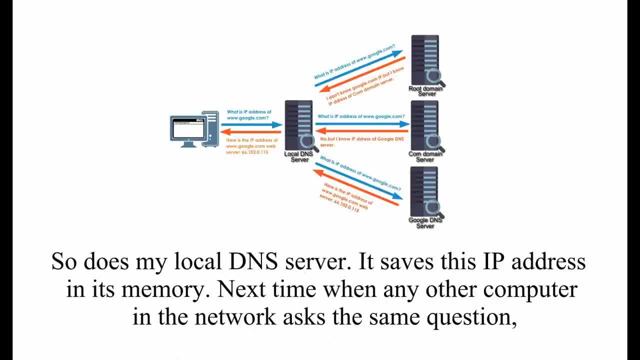 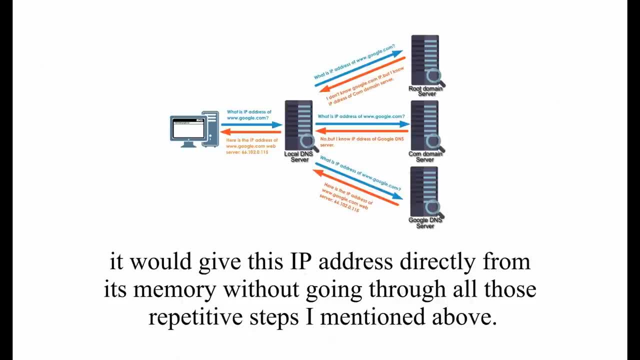 other computer in this network asks the same question and it would give this IP address directly from its memory without going through all those repetitive steps I mentioned above. In summary, DNS requires a lot of time and effort, but you can use your computer to solve. it in a short time. That's all I'm going to talk about today. I hope you have a good time. In summary, DNS requires a lot of time. If you have no time, you can use your computer to solve any problem. So let me give you an example: If you need a lot of time, you can use your computer to solve any problem. If you don't have a lot of time, you can use your computer to solve any problem. That's all I'm going to tell you today. 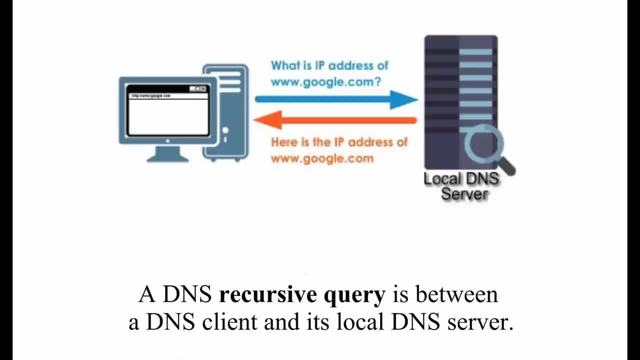 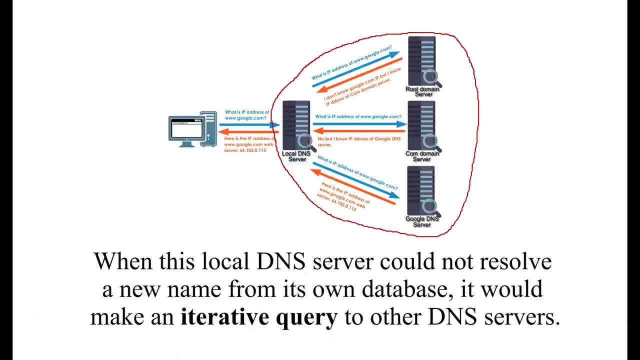 So I hope you have a good time. DNS recursive query is between a DNS client, which is my computer, and my local DNS server. The local DNS server is responsible for answering the questions from DNS clients. When this local DNS server could not resolve a new name from its own database, it will. 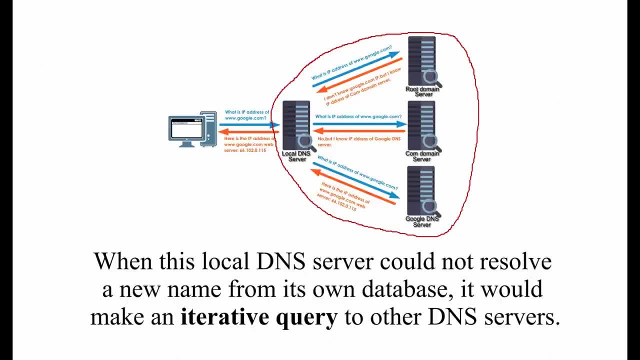 make iterate query to other DNS servers until it finds the answer. I hope this video is helpful. Thank you very much and see you next time.